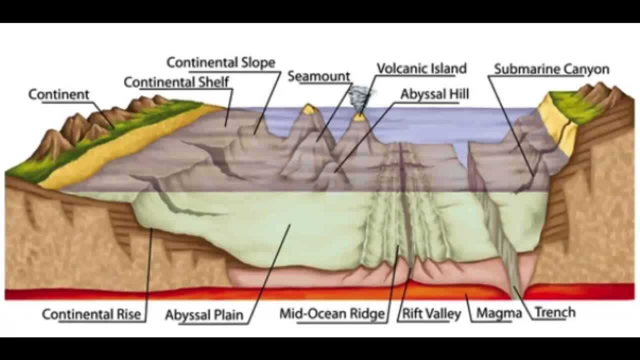 Ocean basins. Ocean basins are large depressions on Earth's surface that are primarily filled with seawater. They make up the majority of the Earth's surface and are characterized by their immense size, deep depths and unique geological features. The ocean basins are divided into five main basins. 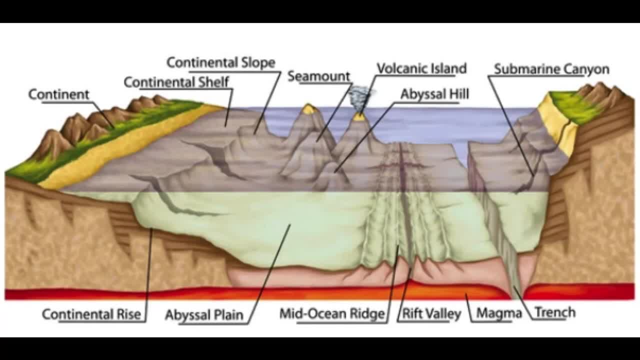 the Atlantic Ocean Basin, the Pacific Ocean Basin, the Indian Ocean Basin, the Southern Ocean Basin and the Arctic Ocean Basin. Atlantic Ocean Basin. The Atlantic Ocean Basin is the second largest ocean basin and is located between the Americas to the west and Europe and Africa to the 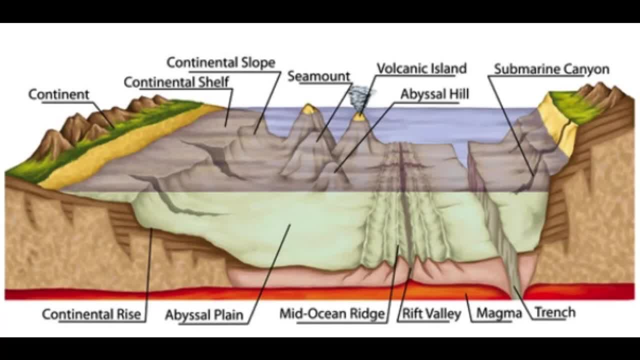 east. It is connected to the Arctic Ocean in the north and the Southern Ocean in the south. The basin is known for its mid-oceanic ridge system, which includes the prominent Mid-Atlantic Ridge. This ridge marks a divergent boundary where new oceanic crust is. 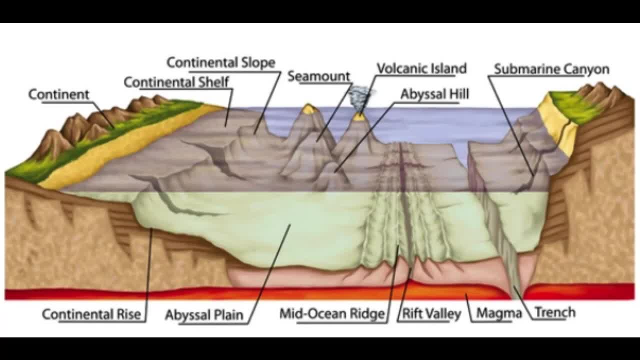 formed. The ridge is known for its wide, wide and wide, wide, wide, wide, wide, wide, wide, and it plays a significant role in the process of seafloor spreading. Pacific Ocean Basin. The Pacific Ocean Basin is the largest and deepest ocean basin. 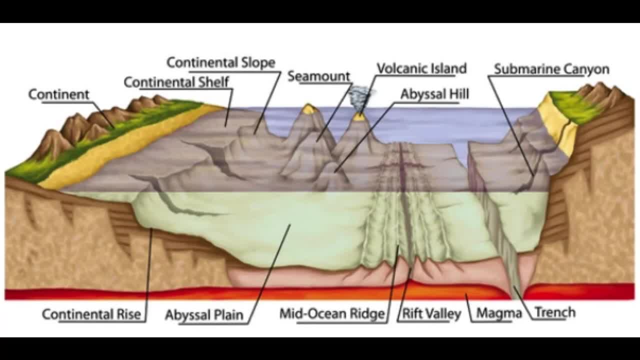 covering approximately one-third of the Earth's surface. It stretches from the western coast of the Americas to the eastern coasts of Asia and Australia. The Pacific Ocean Basin is characterized by the presence of the Pacific Ring of Fire, a zone of intense volcanic and seismic activity. 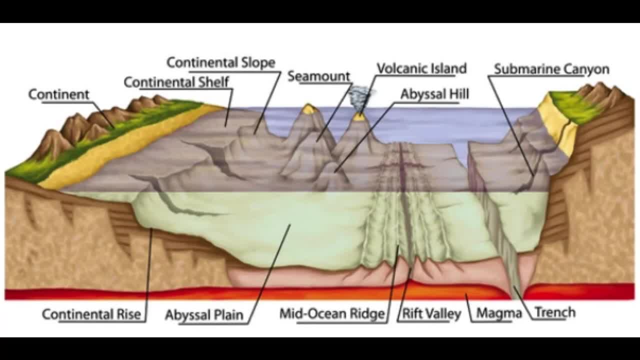 encircling the basin. The basin also features numerous trenches, such as the Mariana Trench, which is the deepest point in the world's oceans- Indian Ocean Basin. The Indian Ocean Basin is the third largest ocean basin and is situated between Africa to the west, Asia to the north. 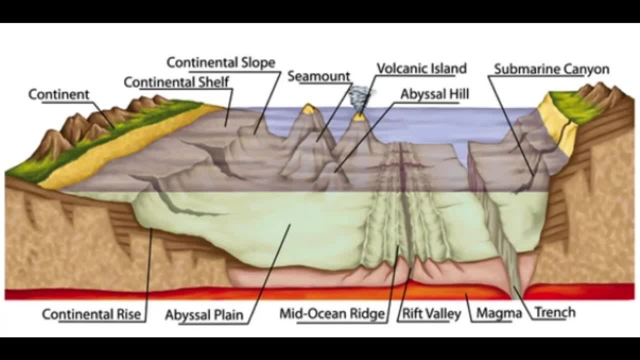 Australia to the east and Antarctica to the south. It is connected to the Atlantic Ocean through the southernmost tip of Africa and to the Pacific Ocean through the Indonesian Archipelago. The Indian Ocean Basin is renowned for its diverse marine ecosystems, including coral reefs, seagrass meadows and mangrove forests. It also contains several